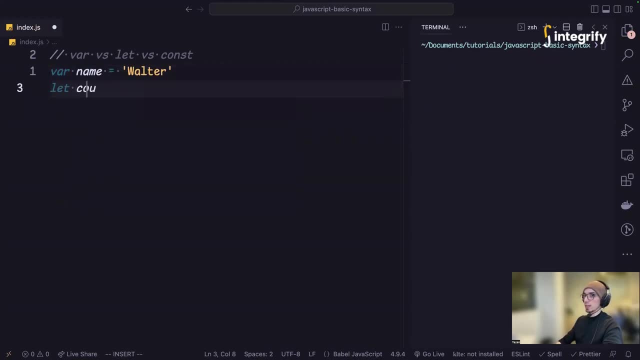 walter, maybe we could. if you want to use lit, we say lit count, for example, and then 12, and then const age is is, is 13 or 30, for example, so it's, the declaration is really straightforward. so you, you declare it with, uh, declared with whatever keyword if you're using varlet or const. 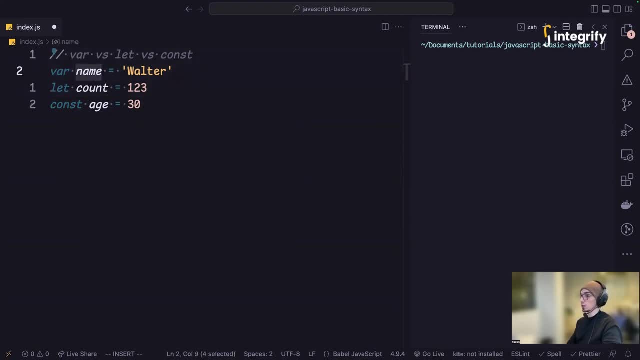 followed by the name of the variable. so you could use it, uh, by the name of the variable. and then we have the assignment. so we assign, we assign it. we assign it to any value, and it could be any type of value, any primitive or reference type. it could be, it could be. 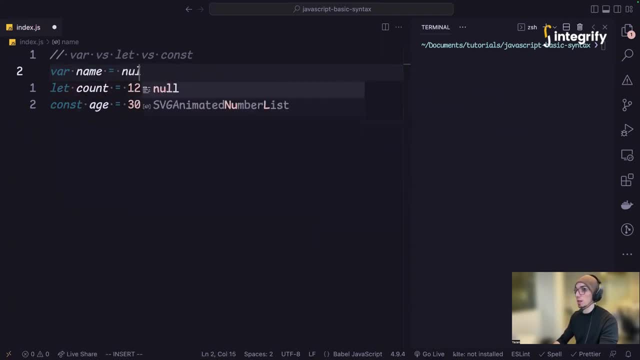 a boolean, uh, it could be undefined, it could be, uh, null, and the list goes on. yeah, so what are the differences? let's see what are the differences and what we can do, uh about them. uh, so, so with var, we can basically uh, let's just say, say, uh, say hi, for example, 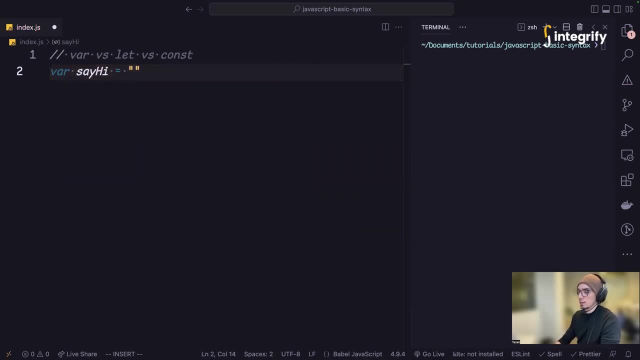 and we can basically just create: let's say hello maybe, and then, uh, if i would basically re declare or declare the value and update it, so say, say hello again. uh, did you see that java or javascript here has no kind of no saying on that? so it's. 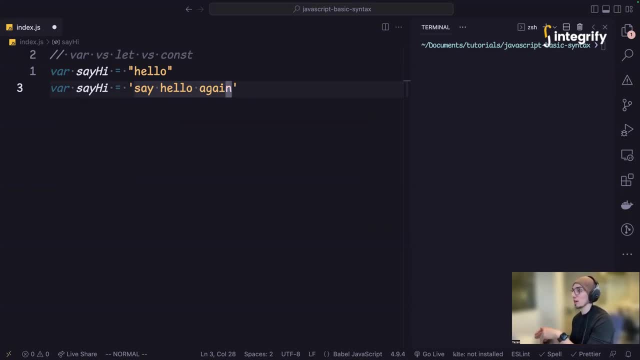 oh cool, do you wanna? you wanna, do you want to create? recreate the same variable, then the same name in the same scope. feel free to do it. i it's. i'm not going to to bother here. if you try to console log uh, console the log the, they say hi, uh. so it's not going to kind of print both of them, it's. 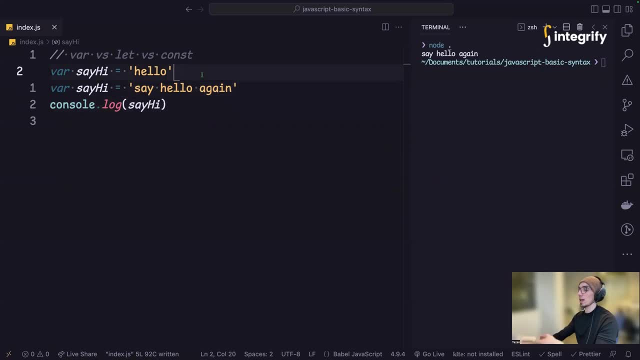 just going to bring the latest one, which is this one, and you can hear, see what kind of bugs it might, might, might you might face later on. which is, uh, what if you? what if you have a long kind of code, like a long file, and you reused or the same name of the variable, and what's gonna happen? 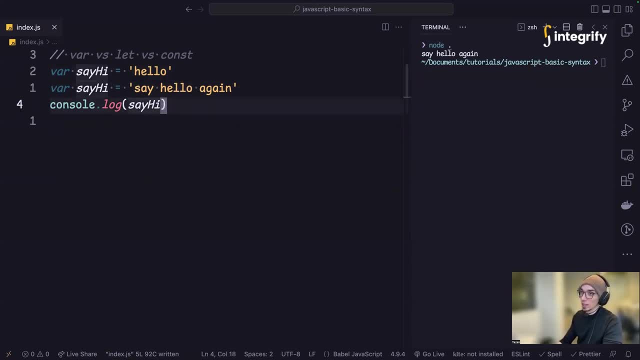 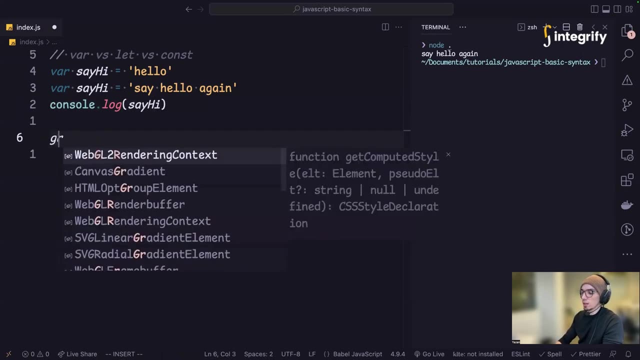 so, uh, it's not gonna be fun at all. all right, so that's one thing here and the other thing with uh, with um, like, if you can go like a greek, like, uh, like a greetings here, and we say, uh, so var, greetings, and we'd say hello, uh, you, and what we could do with var here as well, we can re. 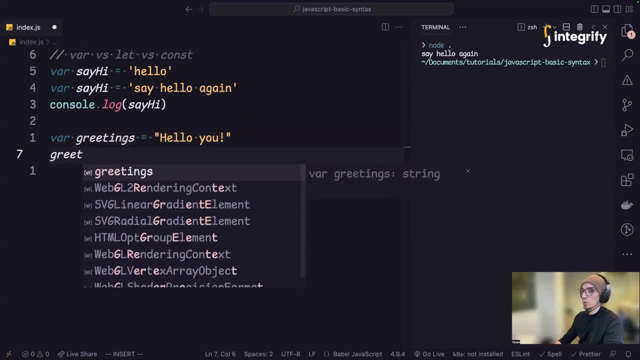 uh, we can re declare the value. so we could just say greetings and we say, uh, hello, maybe i want to decide, i want to say her world. so, uh, we can do those two things with uh with variables or with uh with far and uh, at least for this one here, is just totally fine. but 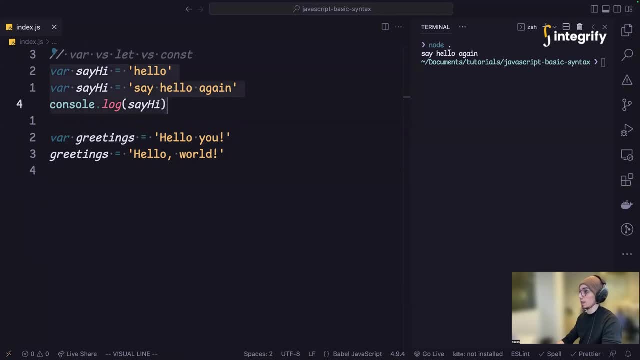 but this one is like the first one, like re-creating, re-declaring the same variable, same name, and without, without any problems. then that's not fun at all. so that's one thing about, about far. so let's talk about, uh, maybe the scope here. what can we? what is that scope? um, so with the scope, uh, let's say you have a. 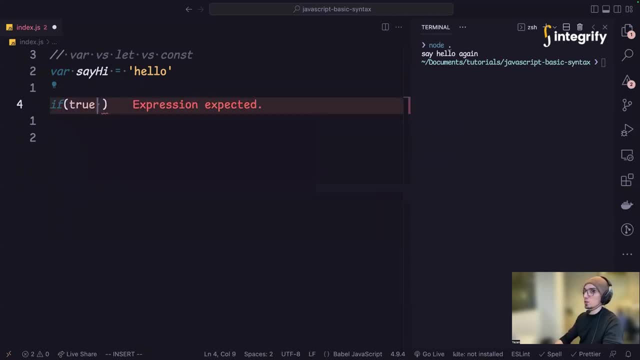 an if statement, all right, and, and the if statement let's say: if it's true, so it will always resolve to true and we're always going to execute whatever here in between the curly brackets. so if it's true, what i want to do is i want to say var, say hi, and so the same name, all right. 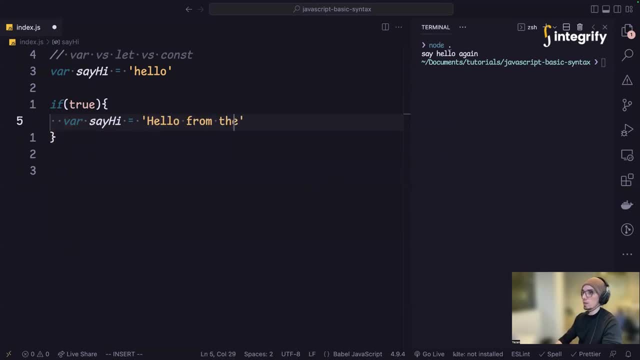 and i will say hello from the uh, from the i don't know inner scope. let's say all right and uh. what else i want to do here at the bottom is i will just consolelog what is say hi. so what do you think the result would be here? is it going to be hello or is it going to be this one? 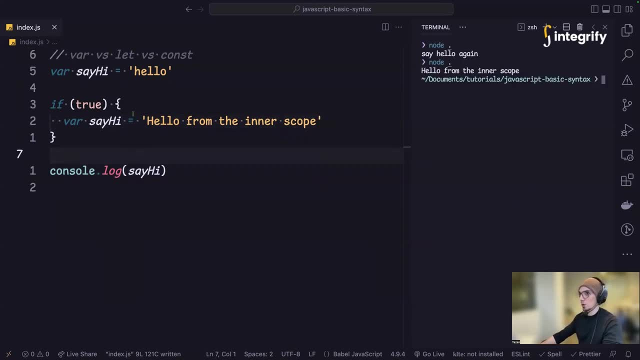 well, if you, you might be shocked with the result, but it's going to actually be that one which is, well, whatever inside this, uh, inner scope, right, it's, maybe you can see here where i'm going, but it's, it's, it's too bad. that's why, uh, it's not recommended to use bar at all, so, uh, the better. 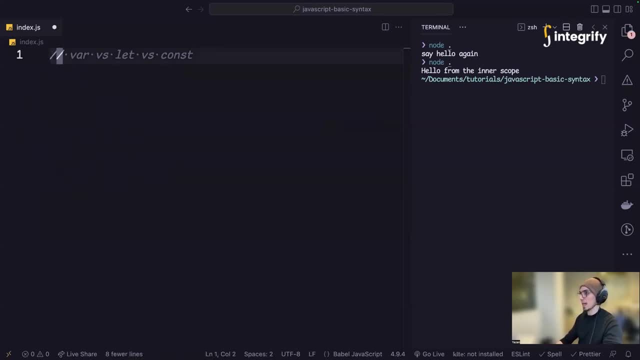 way are uh, var and or, sorry, lit and const. so let's see what is lit. uh, we can easily uh, we can do the same thing with uh. there are like uh, for example, like if you want to reassign, let's totally fine with it, but let's see about uh redeclaring. 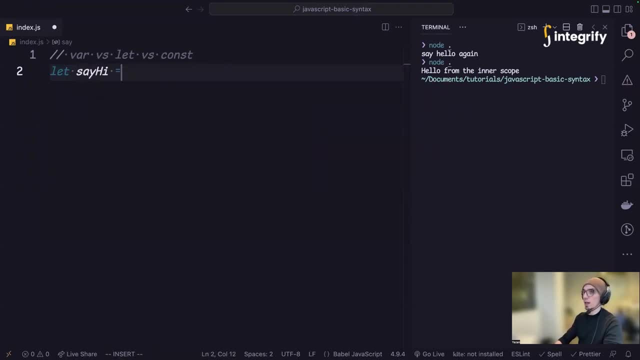 so if i would say, if i have a variable called say hi, and i will say here hi, and then later on i decided: say okay, i'm going to also have an the same variable name but with something else- uh, hi, like that, so you can read here that it's already start throwing an error. hey, cannot really. 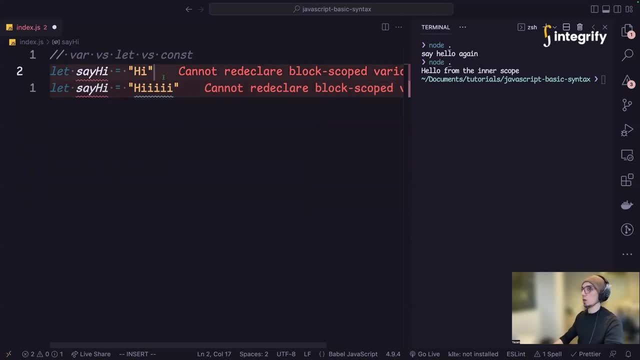 declare a block scope, so if it's in the same block we cannot declare the same name. but what we can do, we can reassign, that's totally fine. we can reassign the value because we can update that value if we want later on. uh, that's totally fine. but if we're going to go back about, about this, 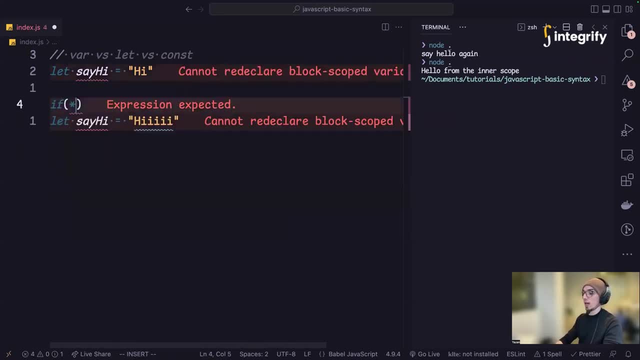 copying issue. what if we have the same example as before? what if i have? if true, and then i basically move this to be inside all right. and if i try right now to to console log, consolelog say: hi, in the previous example we logged this value from whatever inside this, this block. so 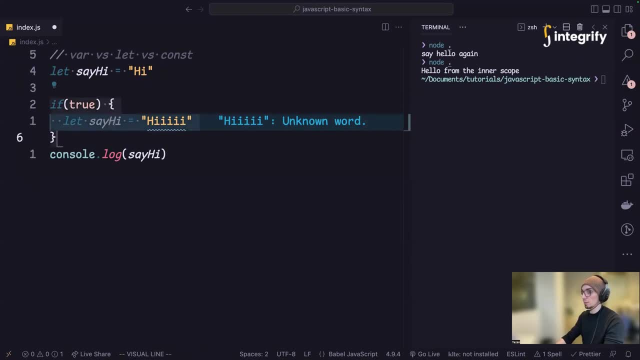 a block is what is whatever here in between the column racks, that's a block, uh. so if i do now save and and run the uh the program again, so you see that it's only printing high, so what do we get from this? so what we understand from this is: uh, first lit can. 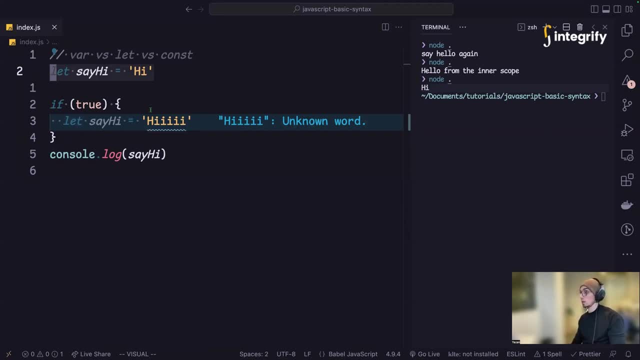 be reassigned but cannot be redeclared. that's one and second. lit is: uh, is a block scoped, so it's only scoped to the plug itself. so meaning that we can use the same name but it must be in a different like, in a different scope, in a different block like. for example, i can have here another like. 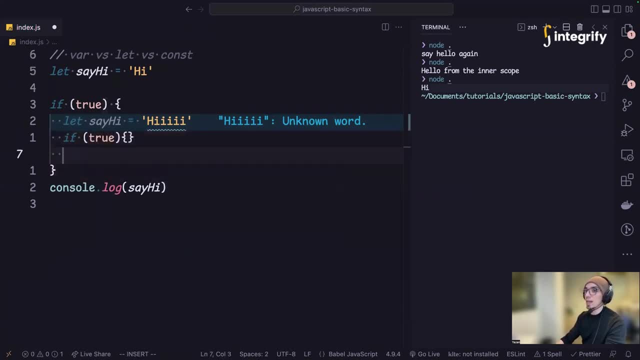 if, for example, and i can also have the same exact name, there is no problem at all with that. i can say: i can have it there and they are all different. uh, they're all different. they are not conflicting with each other. so that's why uh lit is cool. uh, what about cons? uh, const is something that, uh, that. 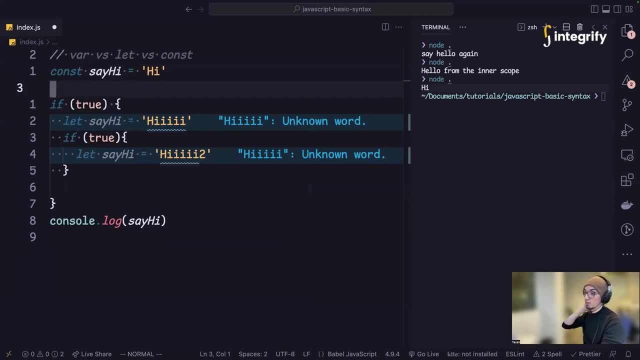 we uh can. it's in. in terms of like scope, it's exactly. it's also a block scope like lit uh, but reassigned value. so i cannot just say say hi and and do something like uh, i don't know. i can't say like hello, for example, word uh. i can't do that with uh, with const. so if i try to, 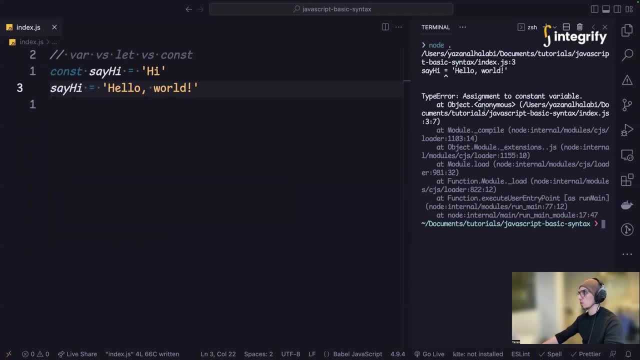 uh, if i try to run the file here, you see that it's throwing an error. i cannot reassign to a constant variable. that's kind of the only difference here, uh, so so yeah, this is this: the var versus lit versus cons. these are the differences and and and. now here it's more, more. 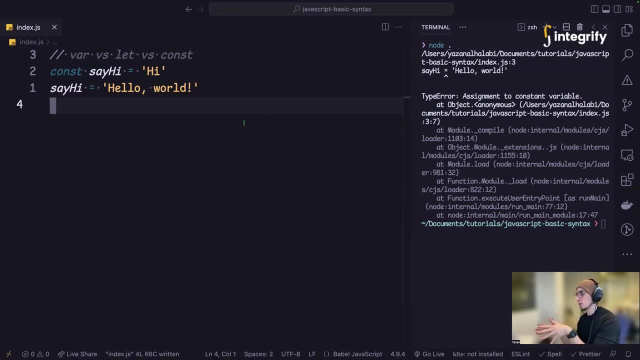 about your uh, either the the team that you're in, what style they follow, or your personal preferences. but for my, in my opinion, my preference is is that i use const as default and then if i want to make that variable to be uh- maybe change later on- or uh, so or i want to. 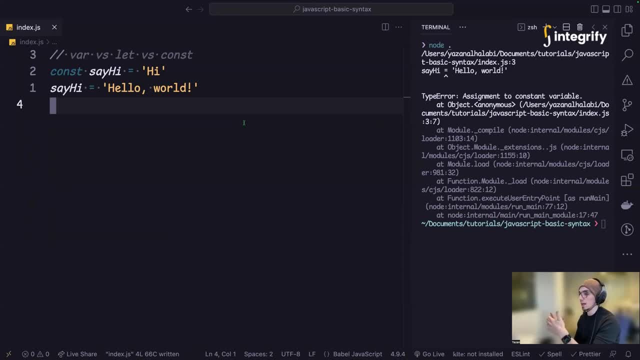 kind of maybe have a counter or a variable that it's gonna. it's gonna change instead value later on. uh, so i would go with lit, but as default i will go with gos. cool, that's it for today. thanks for watching. let me know if you have. 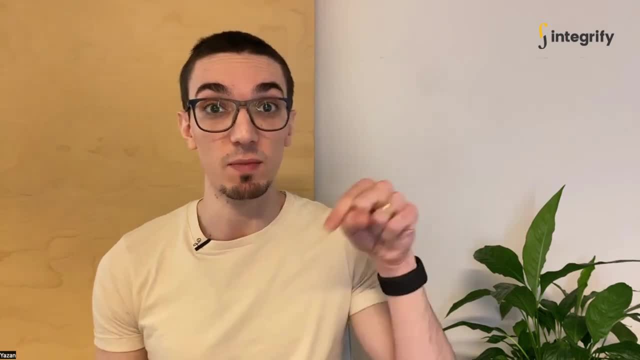 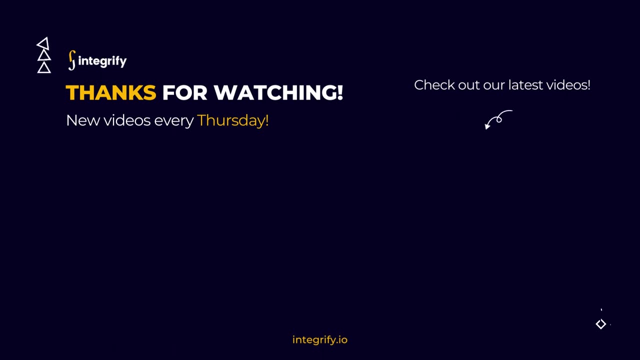 any suggestions or any comments in the comment section below. all right, see you next time.